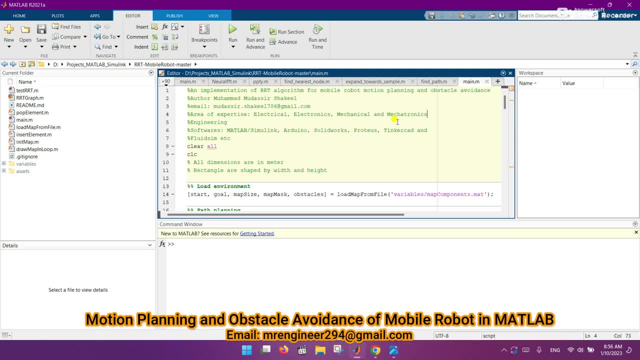 move to the MATLAB scale And let's see the results after running the code. So before running the code, I want to tell you that I am a full-time freelancer in the field of electrical, electronics, mechanical and mechatronics engineering. I have done 500 to 700 projects till now of MATLAB Arduino. 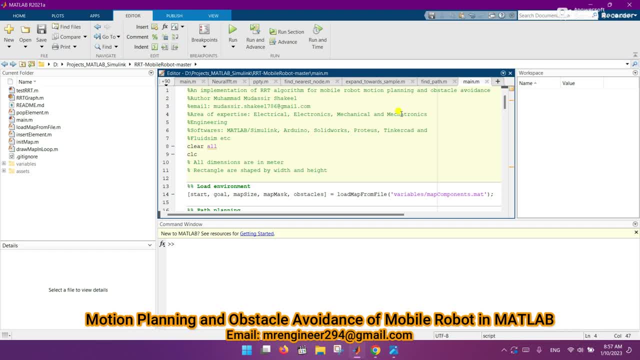 Simulink, Simscape And other engineering software and theoretical subjects. So if you have any assignment, quiz, exam, dissertation, research work of your PhD, MS or Bachelor, then I am ready to help you. So my contact details are given here. My email is this and my WhatsApp number is also in. 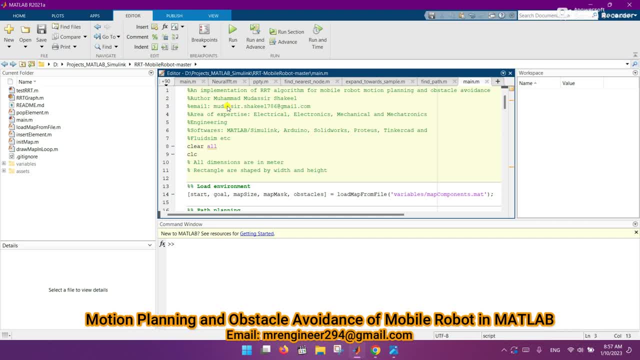 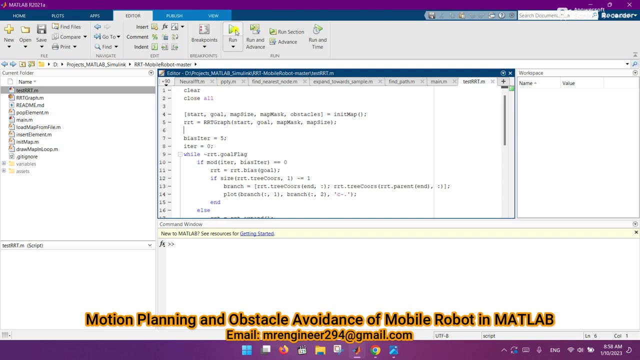 description. You can find me on WhatsApp and email. So let move to the topic of discussion. So let run this code and see the real time results. First of all, let's run the simple RRT algorithm and see the results. Here is the RRT algorithm code. 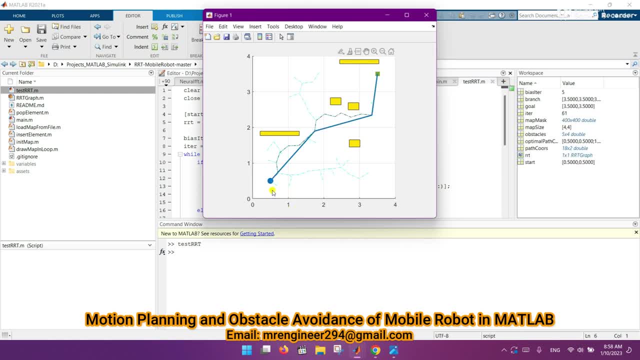 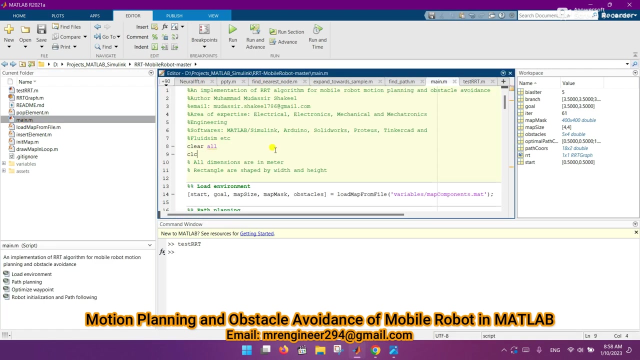 So let me run this code And here you can see that. Here is the graph algorithm. Here is the graph algorithm results of rrt algorithm. that how it, how beautifully it planning up path by avoiding the obstacles. and the second one is for mobile robot. so let's run this main file. 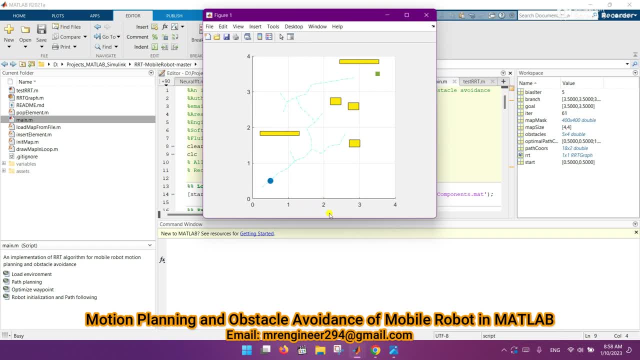 here you can see that here is for mobile robot. now you can see that mobile robot is going toward this goal point by avoiding the obstacle and planning a path using rrt algorithm. you can see that how beautifully it is going to its goal point. and now you can see the. 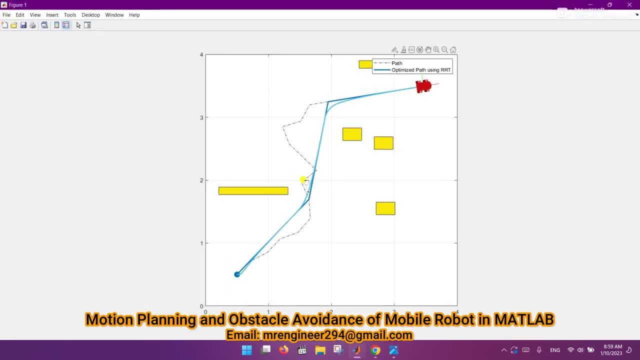 legends of craft that it is the plan. it is a simple path. you can see that it is going to its goal point and now you can see the legends of craft that it is going to its goal point and now you can see the legends of craft that